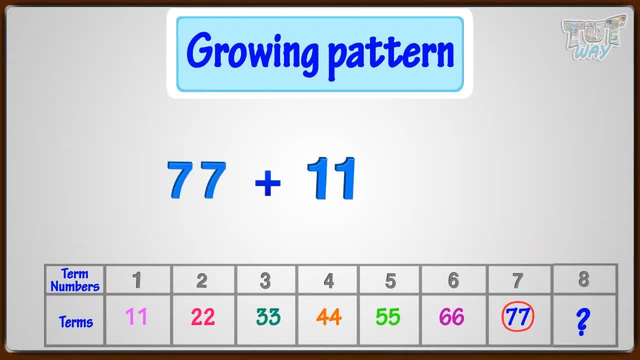 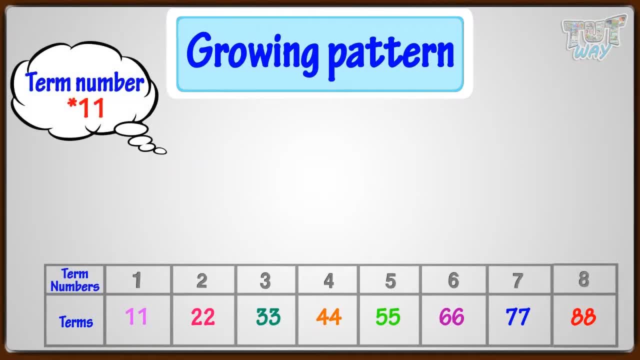 Here we can see that every term is growing. Also, every term is 18 times the sum of June, 2, X, Like the term number one is 11 x 11.. Sir, is absolutely true. isn't slice minus one double? 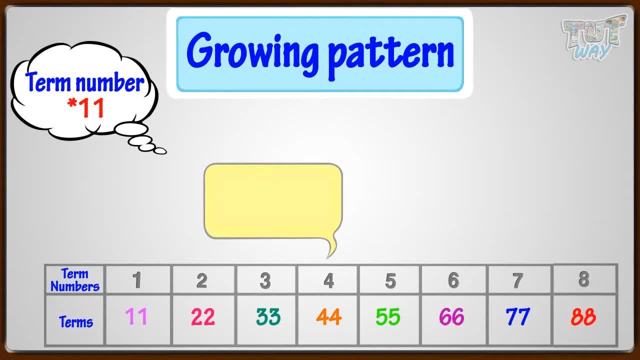 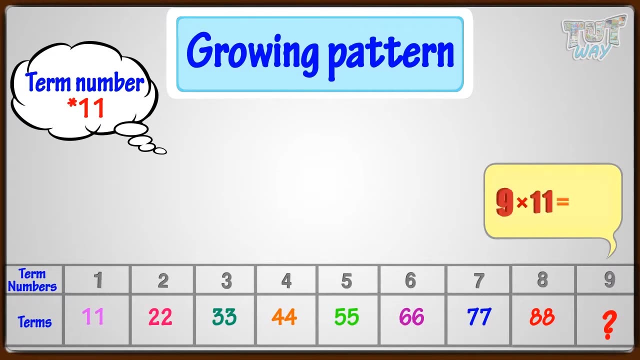 You can also write this in the program. So if you are six, you can say: this is x5.. This isvoila out the ninth term. we can say that it will be 9 multiplied by 11, which is equal to 99.. 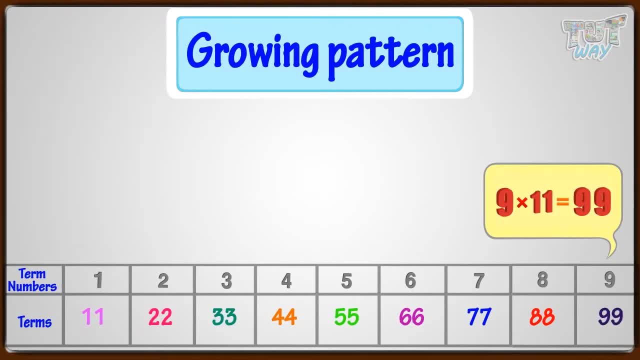 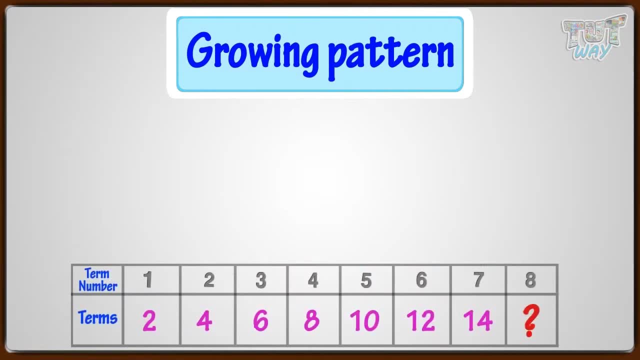 Now let's see more examples of growing patterns Here. what should be the next term Here? we have two ways to find the next term. One is we are adding 2 to every next term. 2 plus 2, we are getting 4.. 4 plus 2, we are getting 6.. 6 plus 2, we are getting 8.. Other, 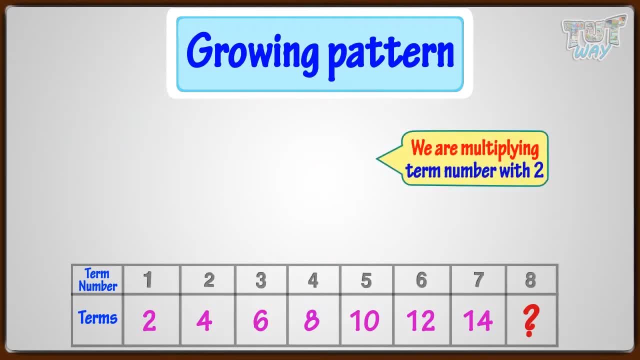 way is we are multiplying term number with 2.. To get the term number 1 is 1 multiplied by 2.. Term number 2 is 2 multiplied by 2.. Term number 3 is 3 multiplied by 2.. Term number 4 is 4 multiplied by 2.. 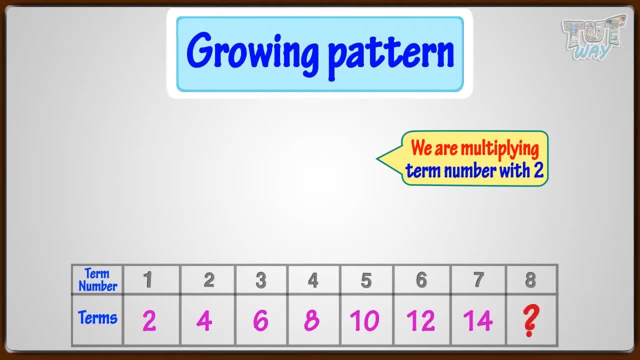 So finding next term or 8th term, here we can multiply 8 with 2.. We can get 16.. Or we can add 2 to the 7th term, That is, adding 2 to 14,. 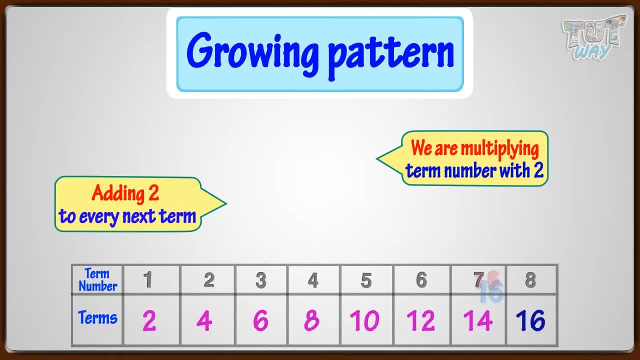 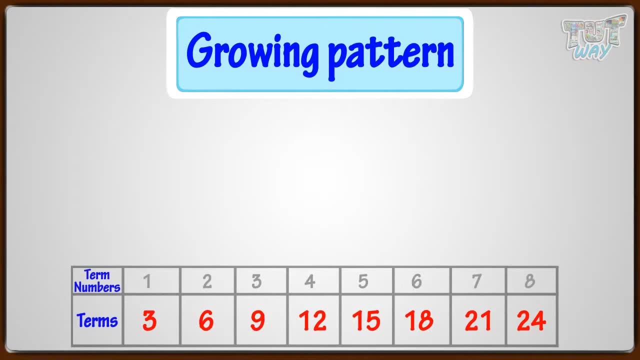 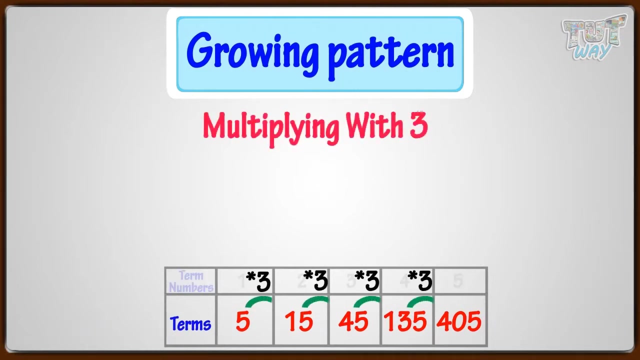 we get 7.. 16. now have a look at more examples of growing patterns. this is an example of growing pattern. here we are adding three with each successive term. here is another growing pattern. here we are multiplying with three. like the first term is five, second term is first term multiplied with three. 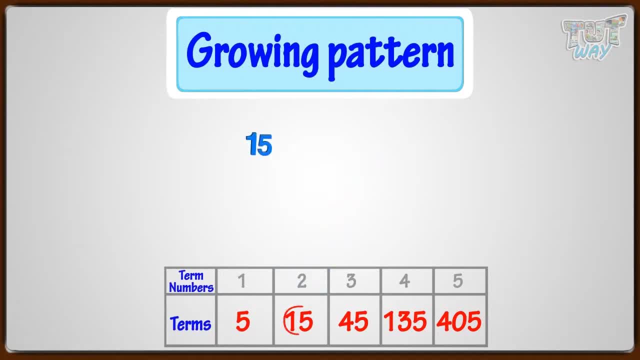 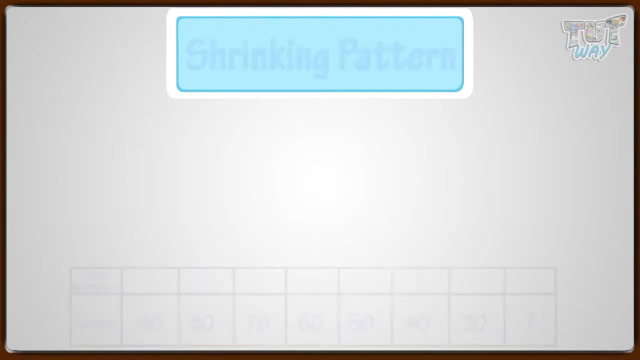 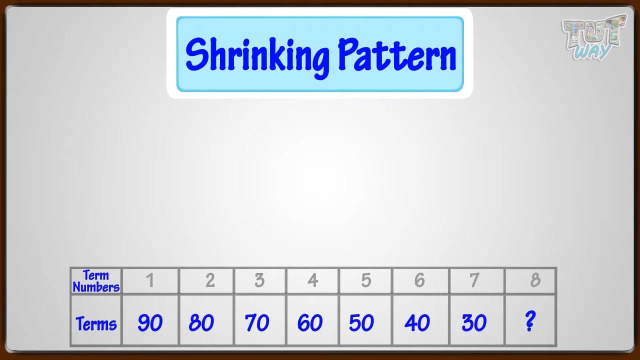 now the next term is 15 multiplied with three, and the next term is 45 multiplied with three, and the next term is 135 multiplied with three. you now let's learn another type of pattern. it is shrinking patterns. here is an example. here the numbers are decreasing with every term, exactly opposite to 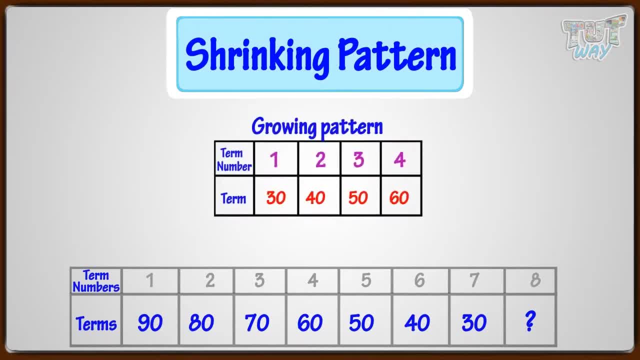 growing patterns where the numbers increase by each successive term. now let's find out what the next terms for this pattern is. here we are subtracting 10 with every term: 90 minus 10, we get 80. 80 minus 10, we get 70. 70 minus 10, we get. 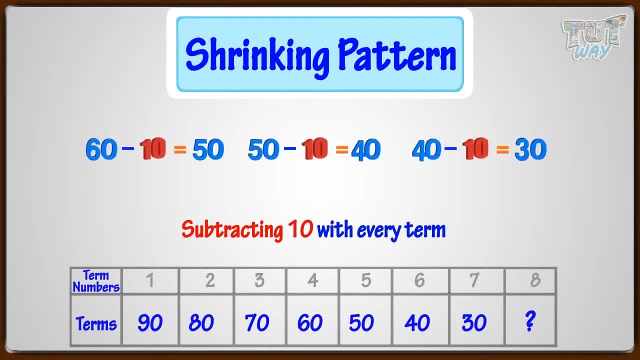 60 and so on. so next 8th term would be 30 and so on. so next 8th term would be 70 and so on. so next 8th term would be 30 and so on. so next 8th term would be: 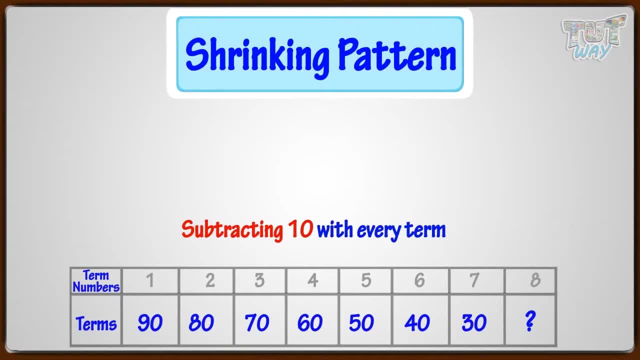 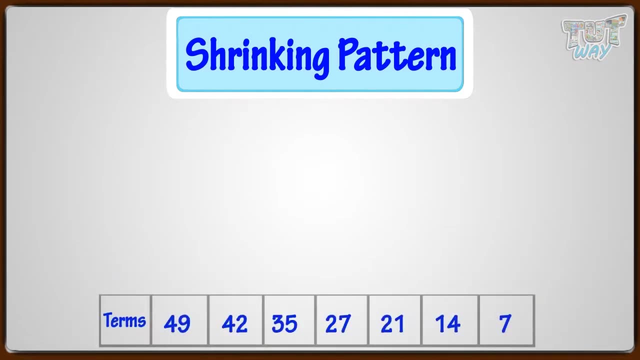 subtracting 10 from the 7th term, 30 minus 10, that is 20. so 8th term would be 20. let's have a look at more shrinking patterns. here we have a shrinking pattern here. what should be the next term? see, here we are subtracting 7 with. 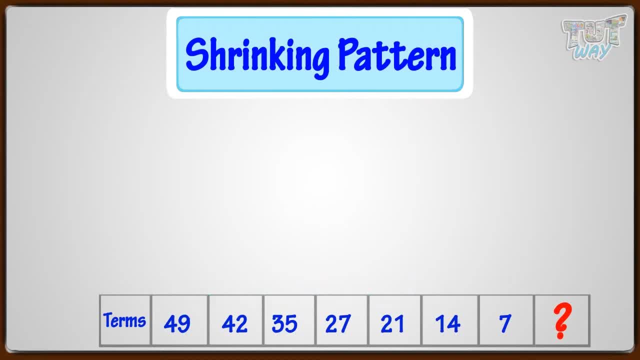 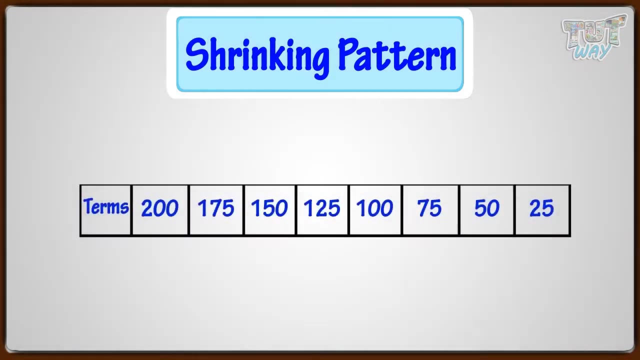 every successive term. so the next term would be 7 minus 7, that is, the next term would be 0. here we have another shrinking pattern. each term decreases with the growing term number. so these are shrinking patterns. let's have a look at some other type of.